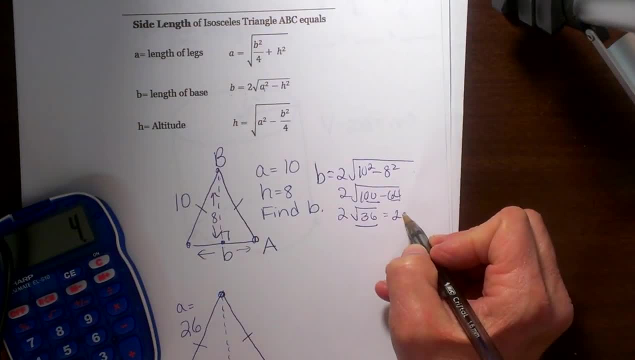 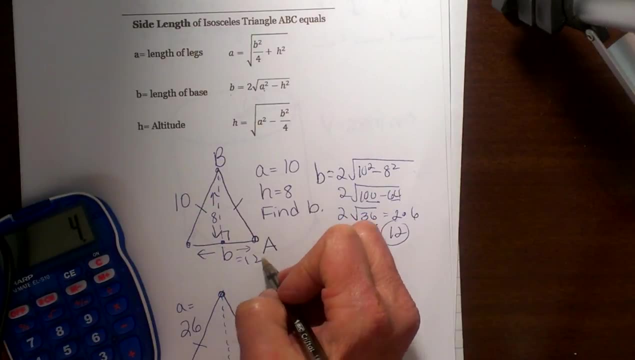 So 2 times the square root of 36 is 6.. So 2 times 6 is 12.. So that is how long my base is down here. So what is this formula? Where is this formula derived from? This formula is actually derived. 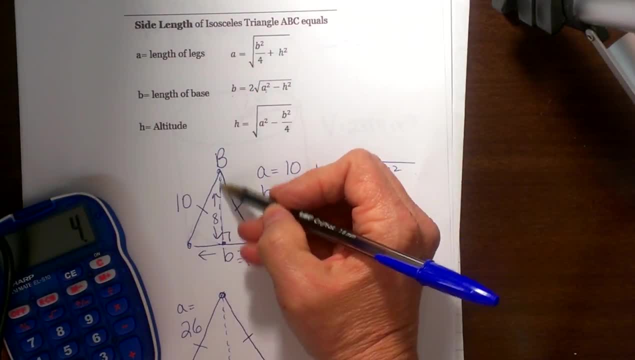 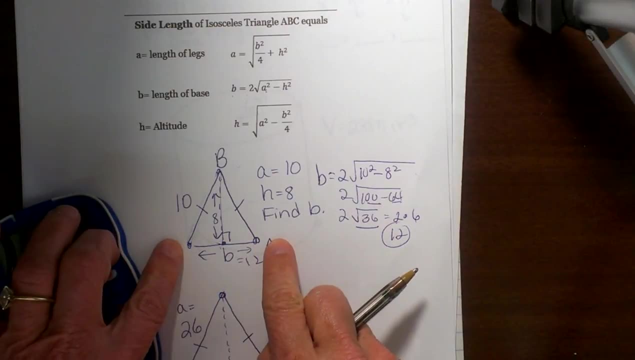 from the Pythagorean Theorem You can see that you have a right side and a left side, You have a right triangle, You have the hypotenuse and you have a leg. so you find the missing leg. and once you find that missing leg, you just double it to find the length of that base. 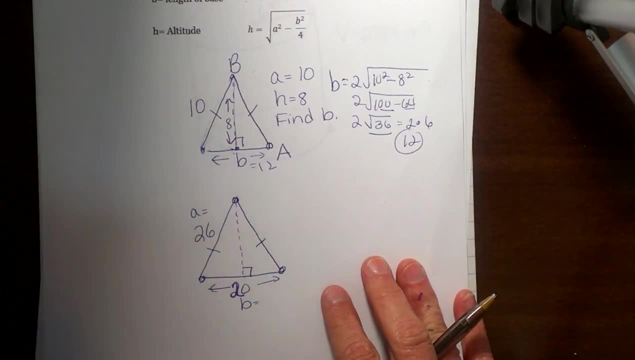 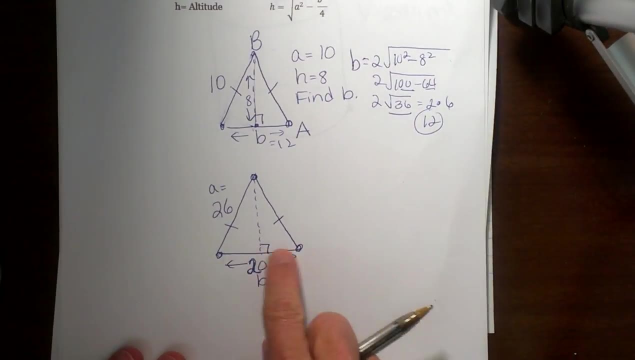 So, just another way to look at it, Let's use our little handy dandy formula to find the height this time. So we are going to use this formula for the height To find this height given the base and one of the legs, and we know those legs are congruent. 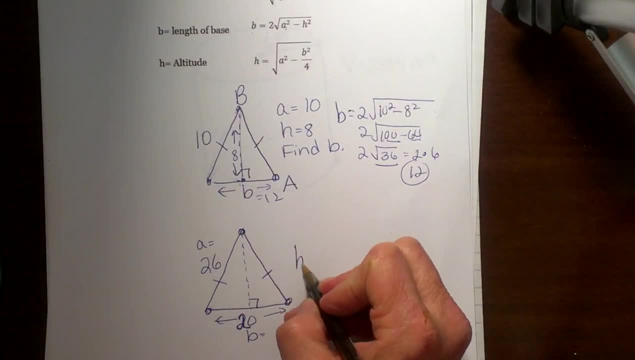 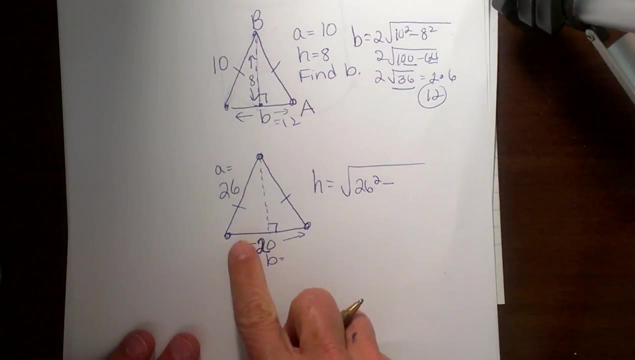 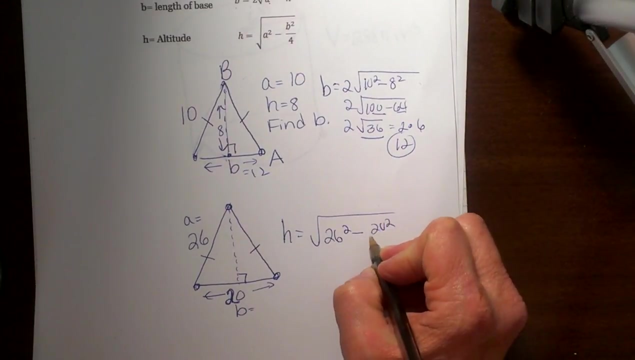 we are going to take. the height is equal to the square root of a squared Well, a is the length of our leg. so that is 26 minus b, squared over 4.. Well, b is my whole base. so I am going to take my base and I am going to square it and then 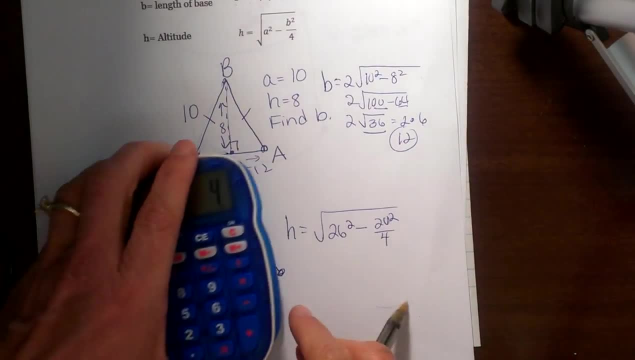 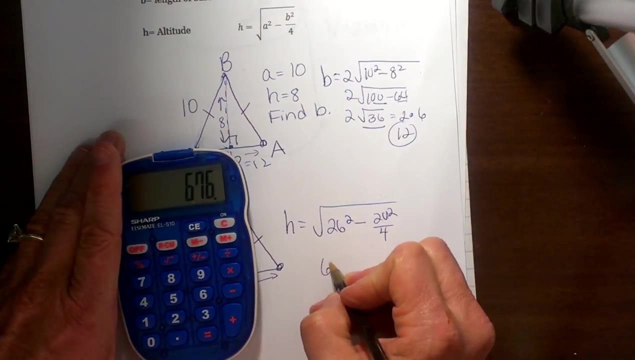 I am going to divide that by 4.. These are some big numbers, so let's do this: 26 squared is equal to 26 times 26, or 676 minus 26 squared over 4.. So 26 squared is equal to 26 times 26, or 676 minus 26 squared over 4.. 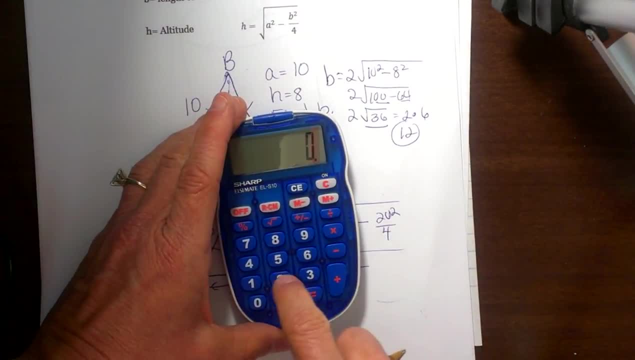 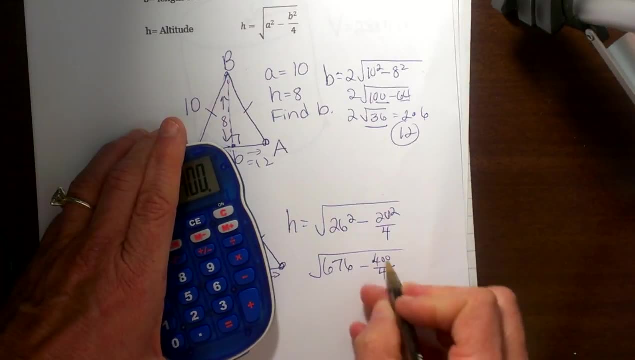 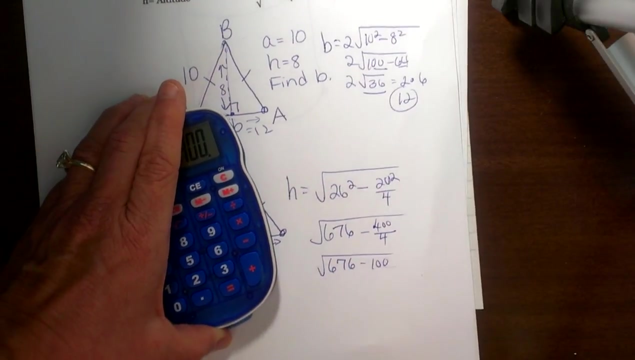 Well, a is the length of our leg, so that is 26 minus b squared over 4.. 20 times 20 is 400, and 400 all divided by 4 is going to give me 100. So let's see 676 minus 100, which is equal to the square root of 576, and that would be. 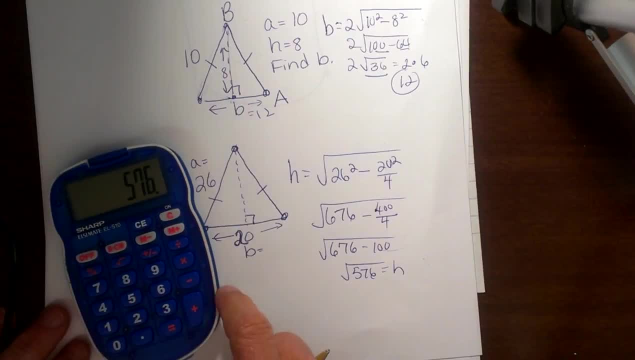 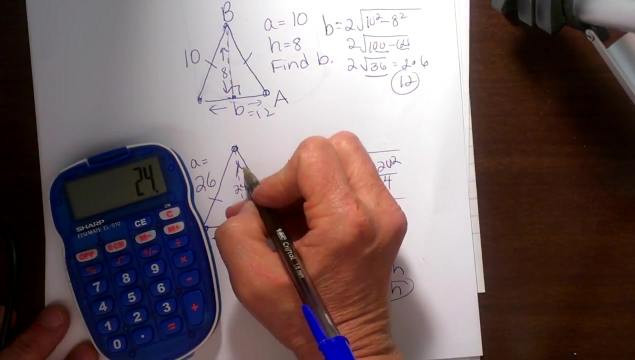 my height. Now let's see if we can't simplify that. That simplifies to just 27.. That is just 24, because that is a perfect square. so we take the square root of that and that means the height is 24.. So the height right here would be 24 using our handy dandy little shortcut formula. I hope this video was helpful.